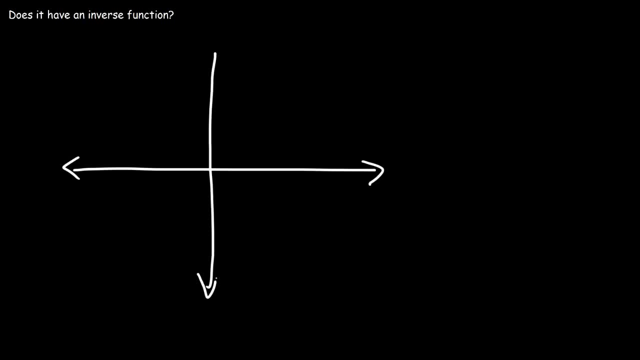 So what about this parabolic function? Does it have an inverse function? Well, if we draw a horizontal line, notice that it touches the horizontal line at two points. So therefore, let's call this function g of x. g of x does not have an inverse function. If you try to draw the inverse relation, it's not a one-to-one function. 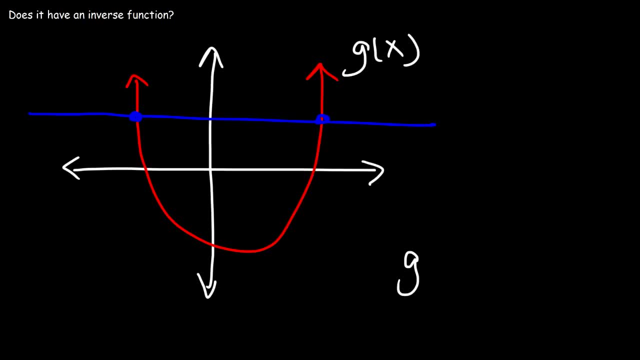 It's not going to be a function. It's going to look something like this: This is just like a rough sketch, And notice that it does not pass the vertical line test. So therefore, the inverse relation is not a function. So we can say that g of x does not have an inverse function. 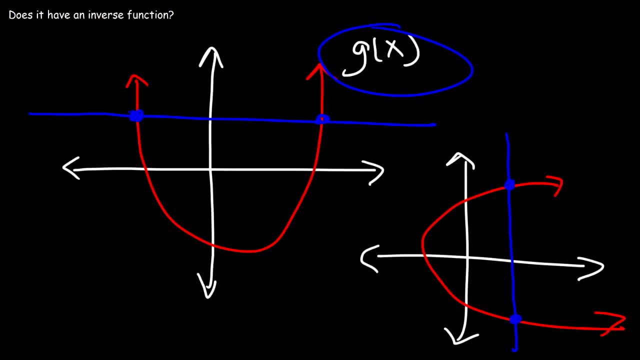 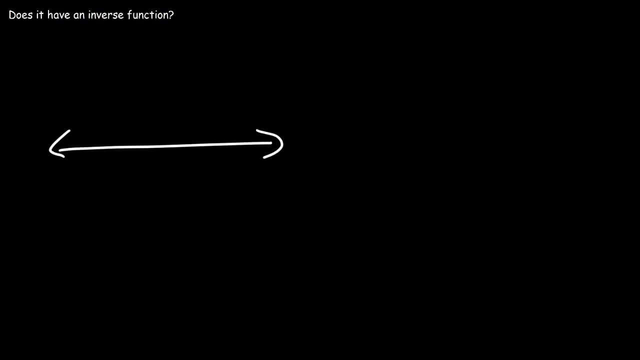 But if we draw a horizontal line, it does not have an inverse function Because it's not a one-to-one function. Let's look at some more examples. So go ahead and determine if the following functions have inverse functions. Let's call this: f of x. 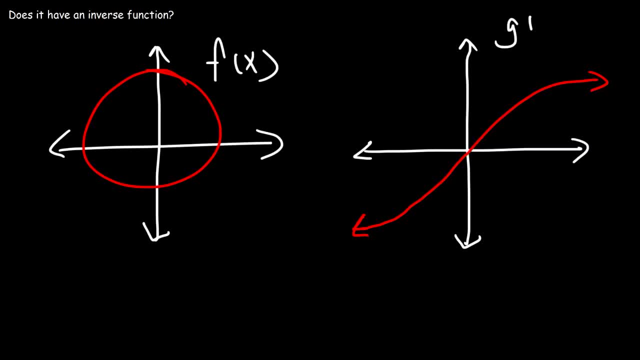 Let's call this one g of x. So f of x does not pass the horizontal line test. It is not a one-to-one function And so it doesn't have an inverse function. g of x passes the horizontal line test. It touches it only at one point. 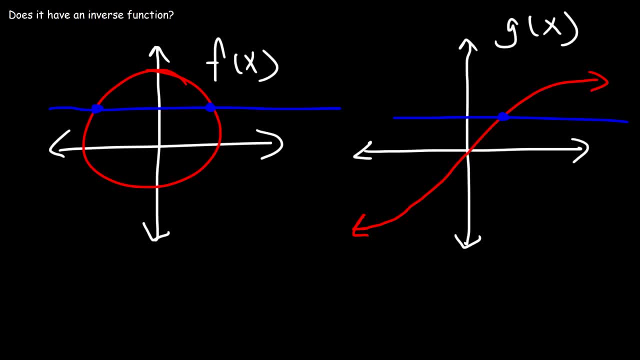 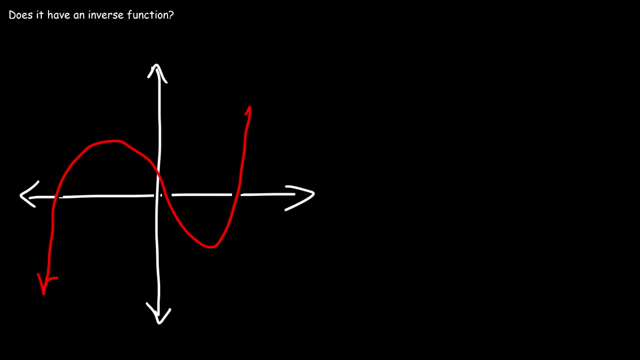 So g of x has an inverse function And it is a one-to-one function. So what about this one? This function does not pass the horizontal line test. It touches it at three points, And so it's not a one-to-one function. 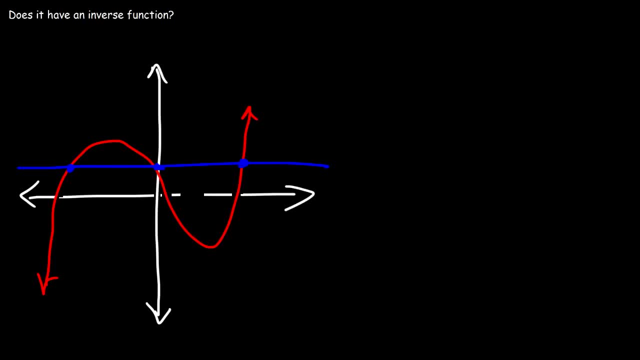 And it does not have an inverse function. So that's it for this video. Now you know how to determine if a function contains an inverse function and if it's a one-to-one function. So keep in mind if you have some function. f of x. 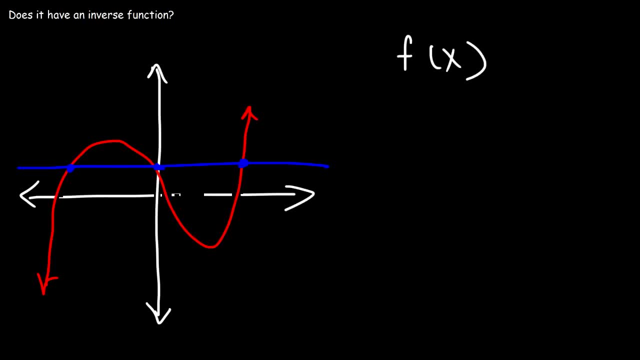 if it's a one-to-one function, that means that it passes the horizontal line test and it does have an inverse function. Let's say we have g of x. If it doesn't pass the horizontal line test, it is not a one-to-one function. 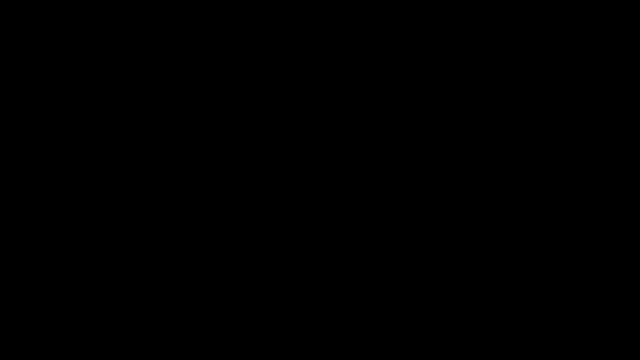 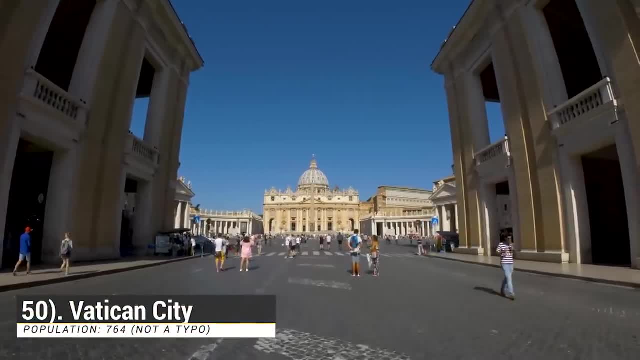 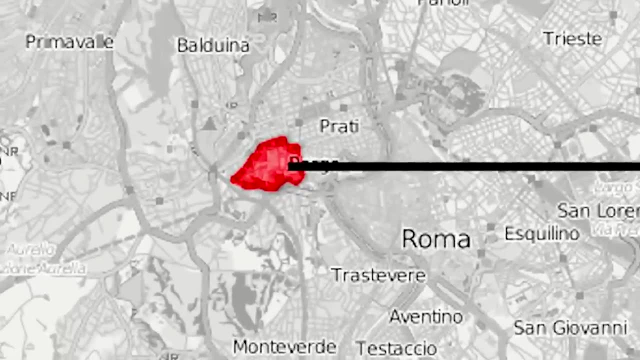 Number 50, Vatican City. At one-fifth the size of Central Park, Vatican City is the smallest nation on Earth, with its entire area located within the city of Rome, And it's obviously last because if you're not part of the Vatican's staff, Swiss Guard, or a Catholic priest or nun, 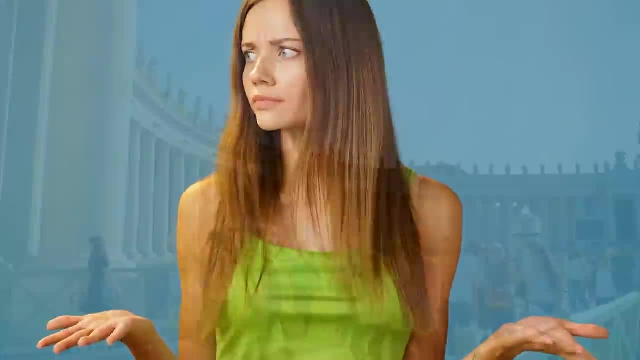 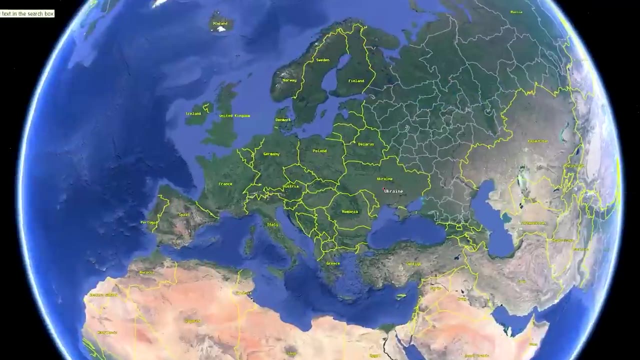 you're not even allowed to live here, But why would you? It's overcrowded, a complete monarchy, and its status as a country is mostly just an excuse to not pay taxes. Number 49, Ukraine. Ukraine is the second largest country in Europe and also home to its second. 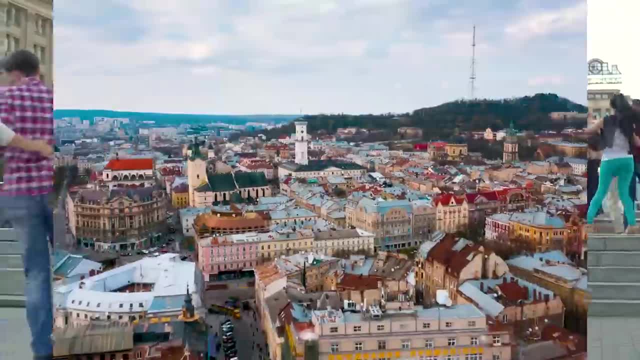 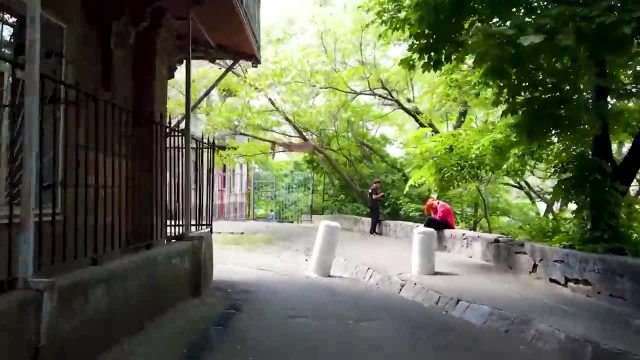 most corrupt government. So, despite its beautiful people, landscapes and history, it's Europe's poorest nation, with a GDP per capita lower than Iraq at $5,200.. The current conflict with Russia has also made many parts of the country not safe. 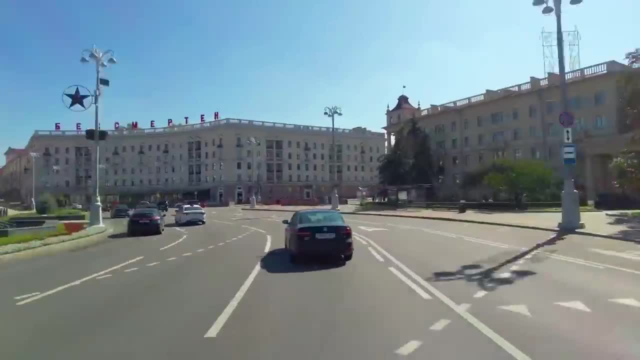 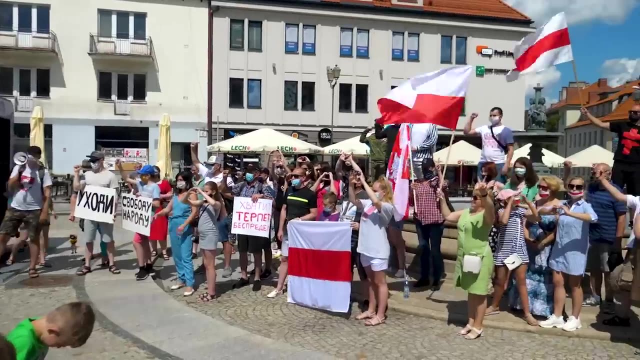 dictatorship. Belarus's president has been in power for more than a decade, And he's been in power for 30 years and routinely invents laws that serve him. Not only is there an extreme lack of human rights, where you'll be arrested and perhaps tortured for peacefully protesting or 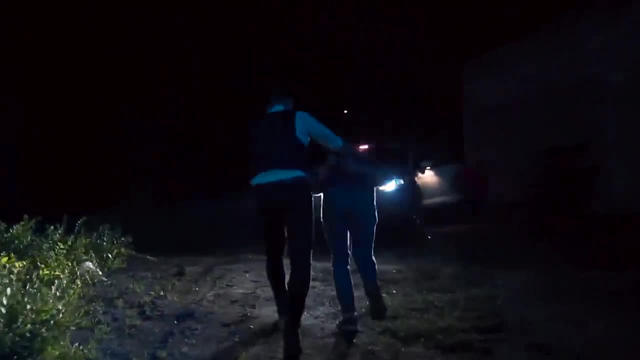 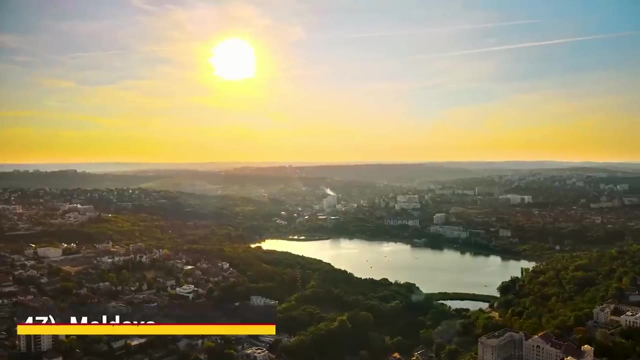 criticizing his government. you can actually be arrested for speaking Belarusian. Yeah, Russian's the official language here. Number 47, Moldova. Moldova is Europe's least visited nation and also its least developed, with the lowest life expectancy.